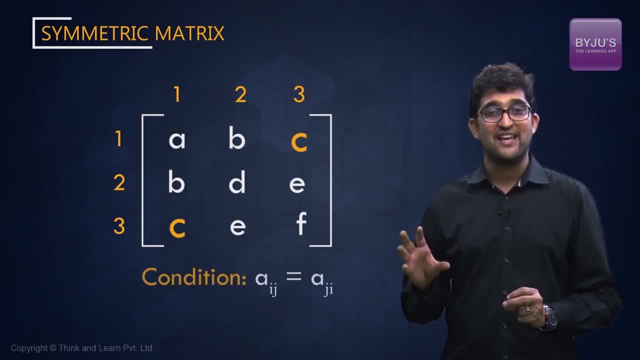 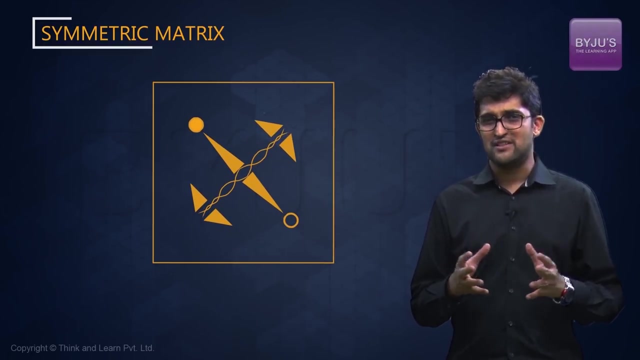 image that Aij is equal to Aji. For any symmetric matrix, Aij is equal to Aji. Let's understand this a little further by taking an image. If I zoom into this particular image, I mean this image obviously is a symmetric image. you go deeper into it, you take a transpose. 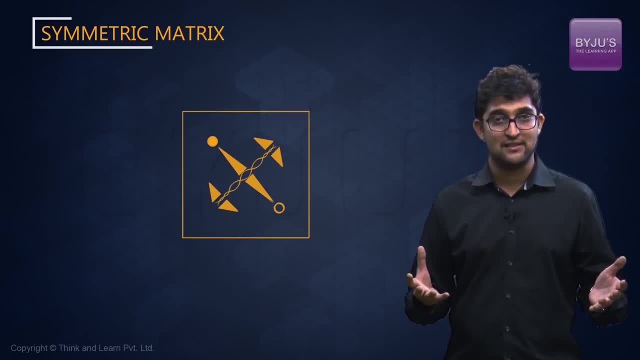 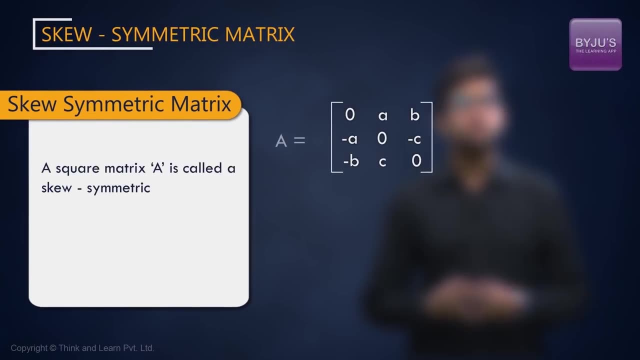 of it. now zoom out again. What do you get? You get the same thing. This is the idea of a symmetric matrix, A skew. symmetric matrix is defined as a matrix in which the transpose of the matrix is equal to the negative of the matrix. That is, mathematically. 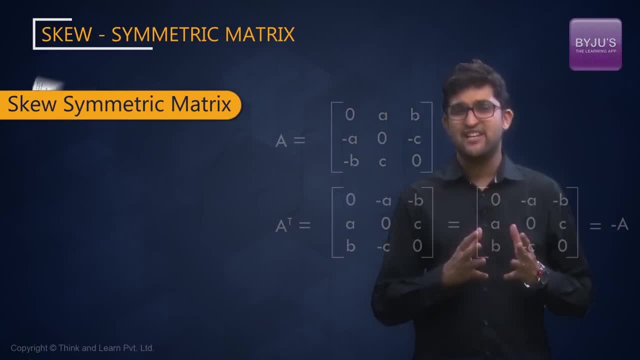 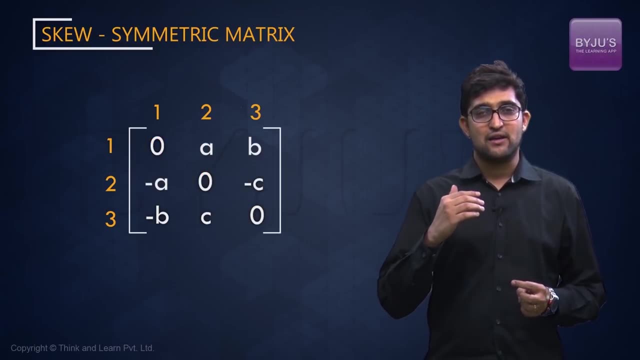 A transpose is equal to minus A. Let's take an example. So in this example, you can observe that you have the diagonal elements, and the elements above the diagonal elements are mirror images of the elements below the diagonal elements, with a twist. What is that twist? 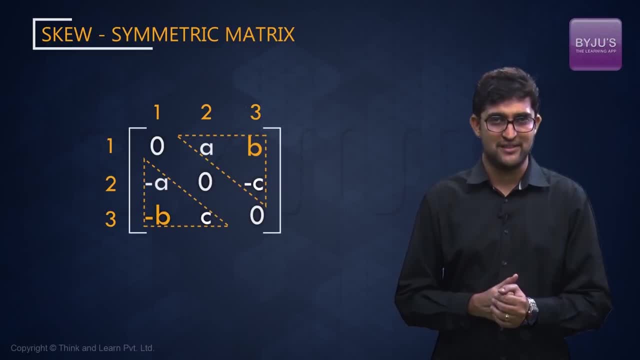 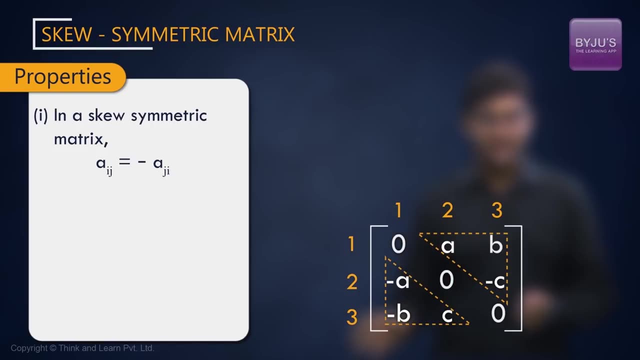 in the symbol right, negative becomes positive and positive becomes negative. so fundamentally I can say that in a skew symmetric matrix, aij is equal to minus aji. so in any skew symmetric matrix- this is the property- aij is equal to minus aji. what is the second inference you can draw from here? the? 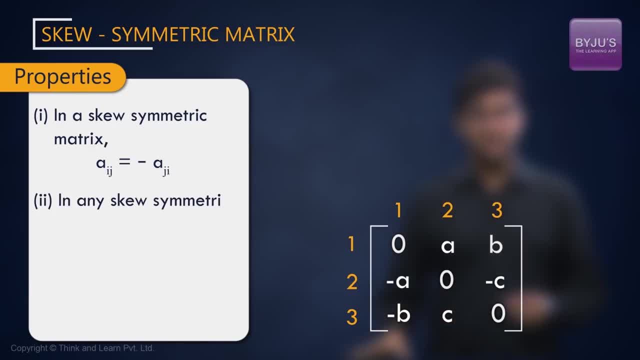 second point about skew symmetric matrix is: in any skew symmetric matrix, all diagonal elements are 0. this will work out with respect to the first property also, because you are seeing, aij is equal to minus aji. that means a11 is equal to minus a1, which is the only value possible: 0. now that we 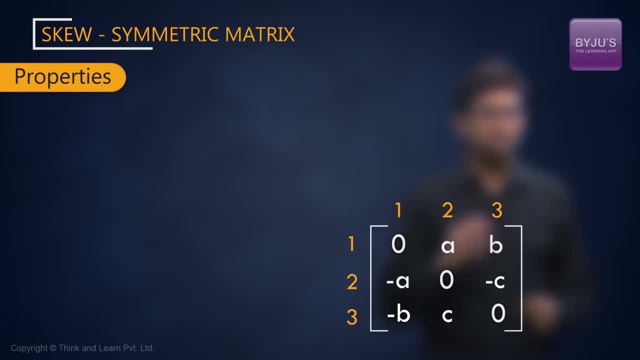 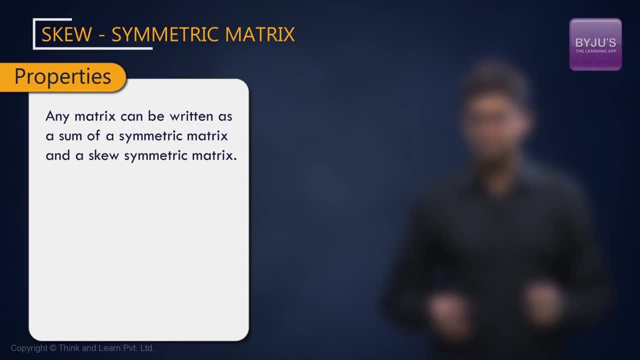 have learned symmetric matrix and skew symmetric matrix. here is a quick fact for you. any matrix can be represented as a sum of symmetric matrix and a skew symmetric matrix. how? let me explain. you have a matrix A. I can write it as A plus A, transposed by 2 plus. 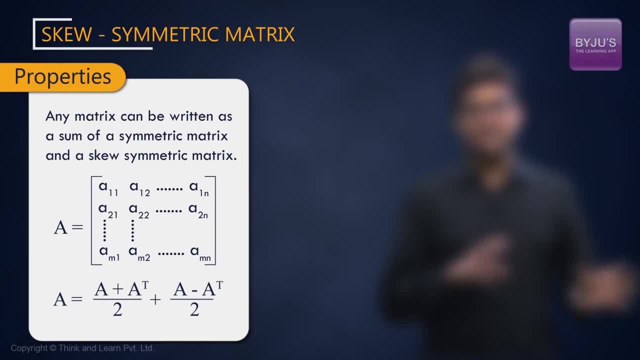 A across the body, A piece a and a plus Rx as well. I can write it as A plus A, transpose by 2 plus A. let me explain. you have a matrix A. I can write it as A plus A transpose by 2, plus A minus a transpose by 2. so a is written as a combination of two matrices. look carefully at. 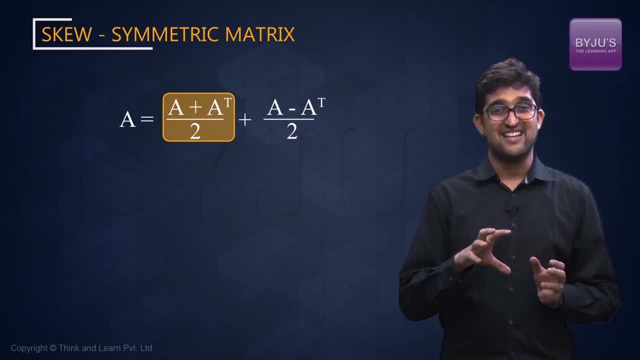 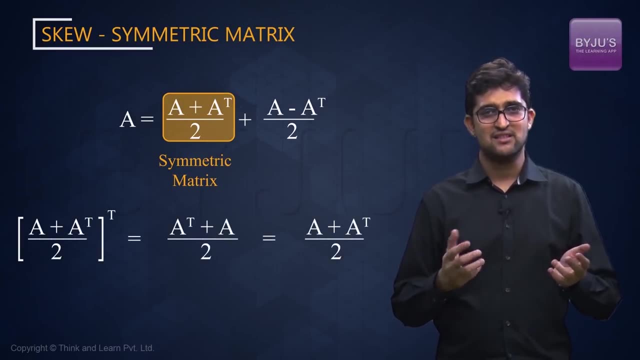 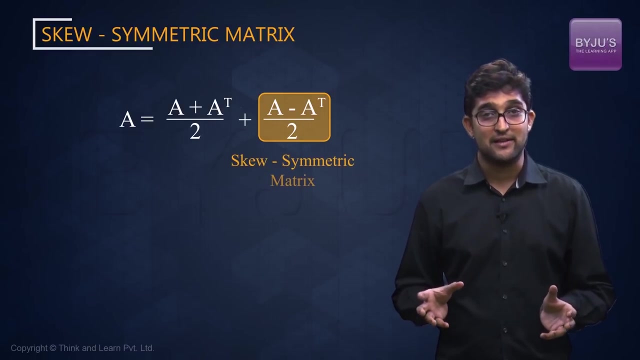 this: a plus a transpose by 2. this matrix is a symmetric matrix. why is it so? take the transpose of it. what do you get? you get a transpose plus a by 2, same as earlier. yes, so this is a symmetric matrix. now look at the other one: a minus a transpose by 2. this is a skew symmetric matrix.